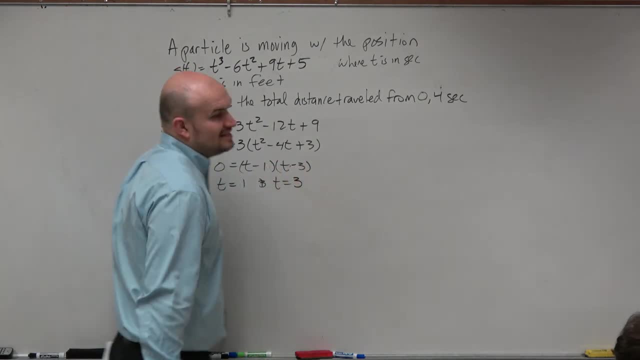 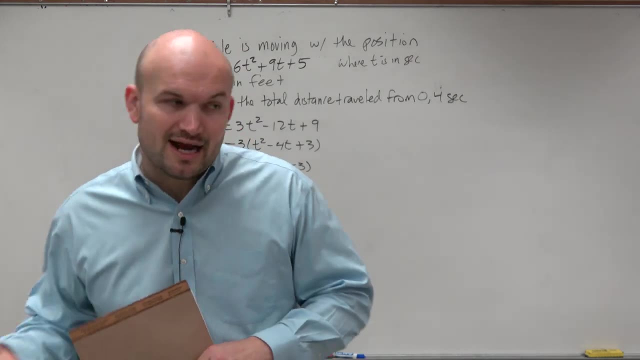 am I doing? That's negative 3, right At t equals 1 and at t equals 3, the particle is potentially changing direction, right, And obviously we could justify that it's changing direction by actually plugging in a test point, right? Can we plug in like: 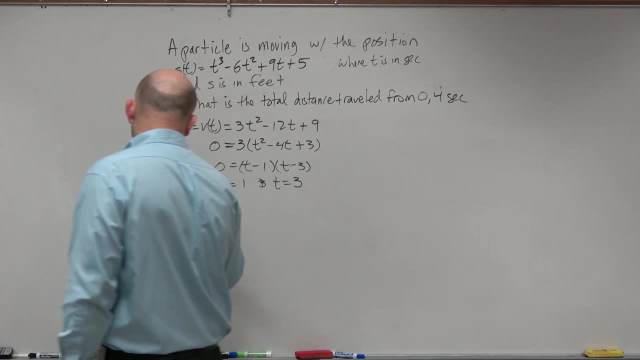 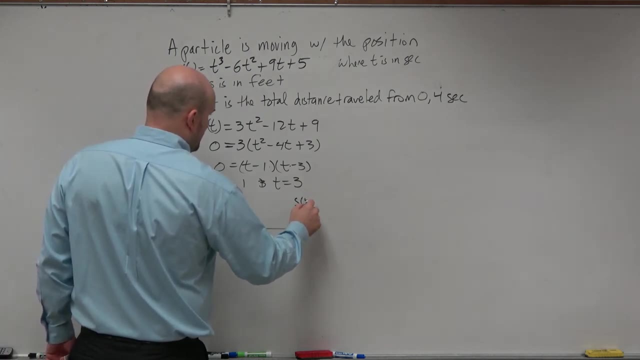 between zero is the initial point. So if we draw a like kind of number line here, So here we have s of zero, which is like the beginning, Here we have s of 4, which is the end, Then we 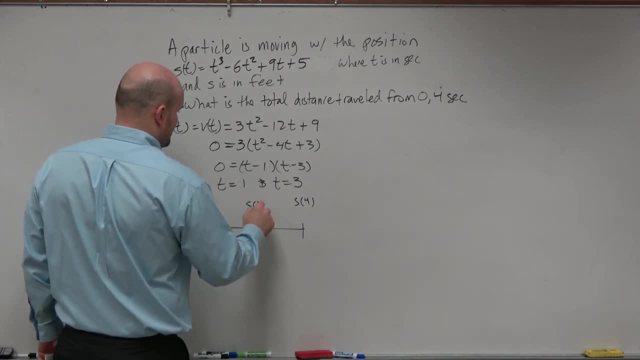 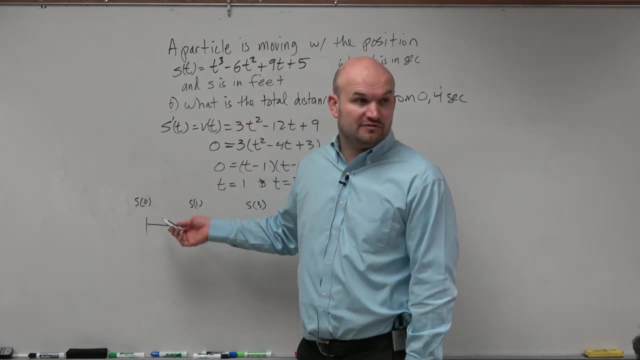 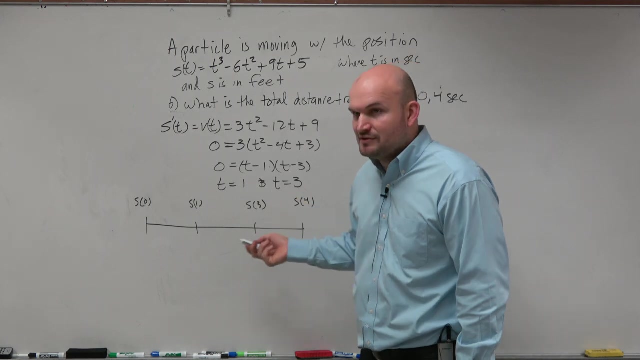 have s of 1, and we have s of 3,, right, And obviously, ladies and gentlemen, we could plug in points like s of one half to determine if the velocity is positive or negative, plug in s of 2 to determine if it's positive or negative, and determine like s of 3.5 to determine. 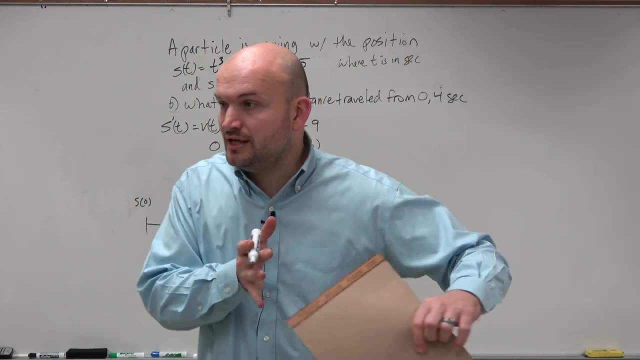 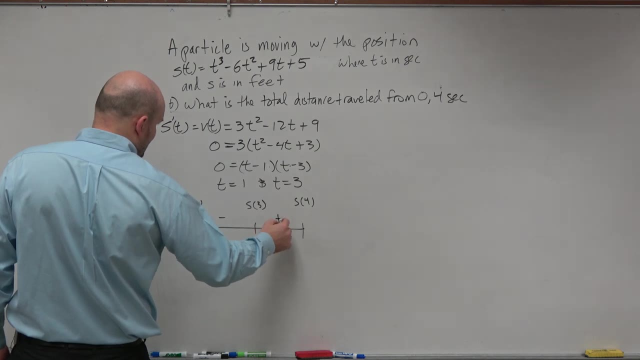 if it's positive or negative, And that's just to verify if it's going to be changing direction at those points. And to look at it, actually, that's going to be positive and to negative and then back over to positive if you were to go ahead and plug those in. But in the 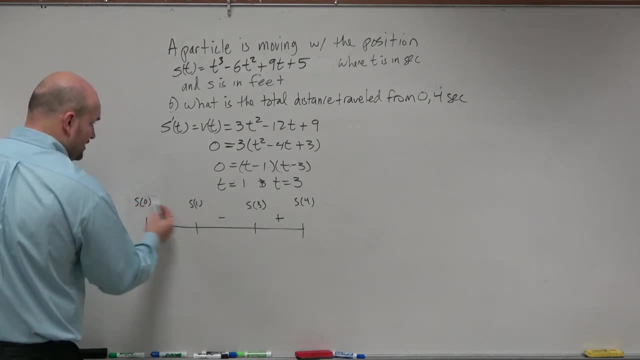 reality. the main important thing we want to do is find the change. How far did it change from s of 1 to zero? It doesn't really matter if it's positive or negative. in this case We've got to find the distance traveled here, So we're going to take the absolute value. 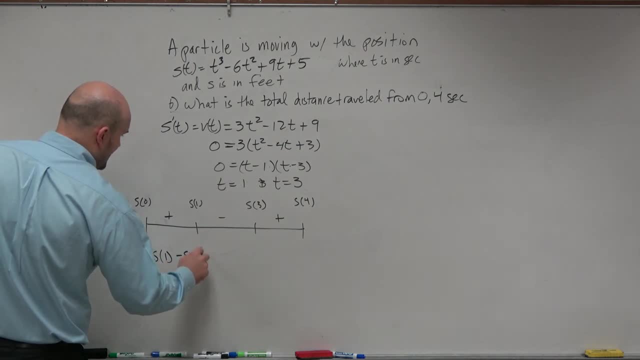 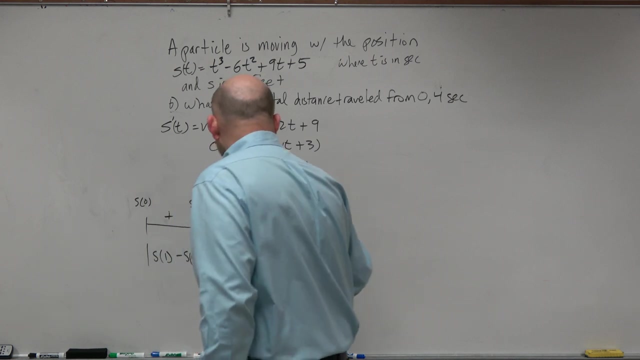 of s of 1 minus s of 0. That is showing the displacement from 0 to 1.. Does that make sense to everyone? And then we're going to add that to the absolute value of the displacement from 0 to 3 to 0 to 1.. And then we're going to add that to displacement from s of 4 to. 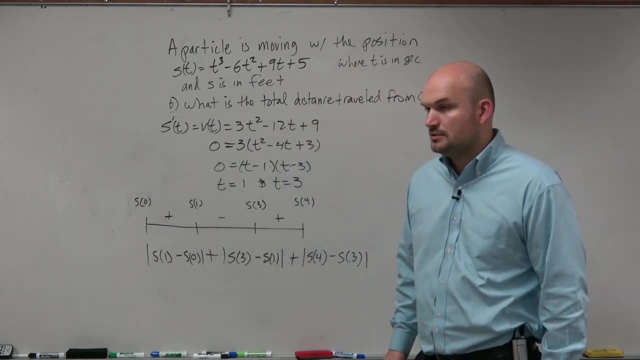 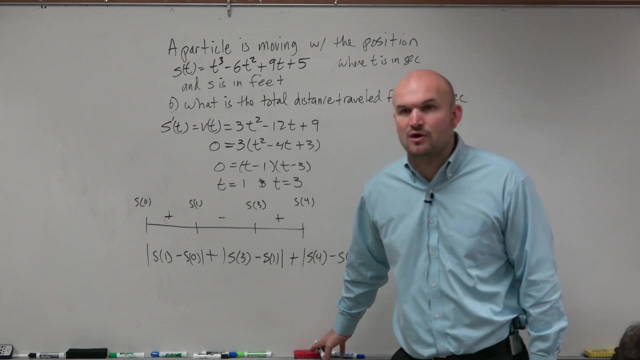 s of 3.. Does everybody see what I at least wrote in there? Does that make sense? Because if that makes sense, then the only way that you would have got something wrong is if you just made some arithmetic errors, Because from here, this is the main idea- is: 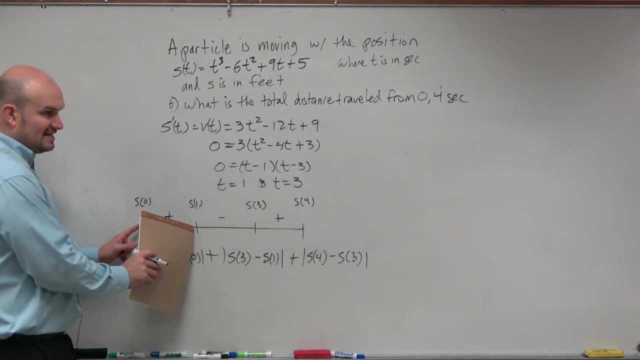 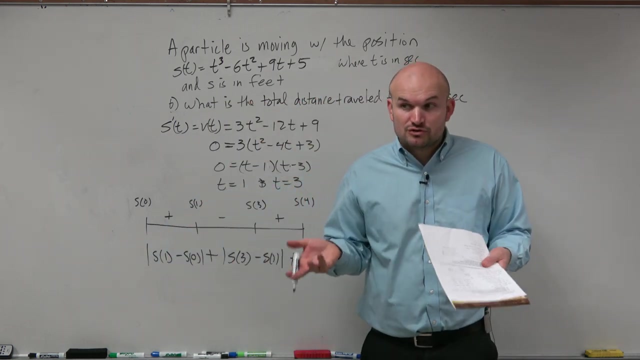 understanding that, even though it's changing direction, you're finding this distance plus this distance, plus this distance by finding the displacement using subtraction and then the absolute value, taking away the direction, Because we don't really care about the direction, We don't care if you go four miles this way and four miles that way, You still traveled. 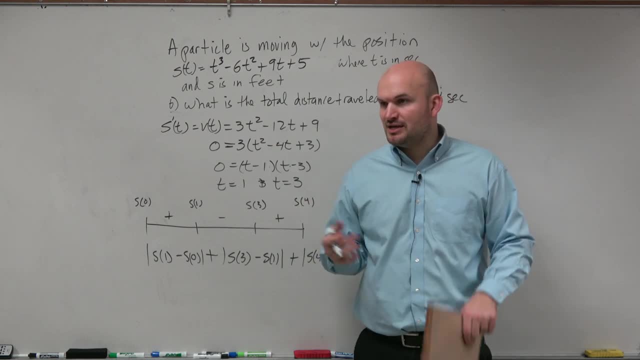 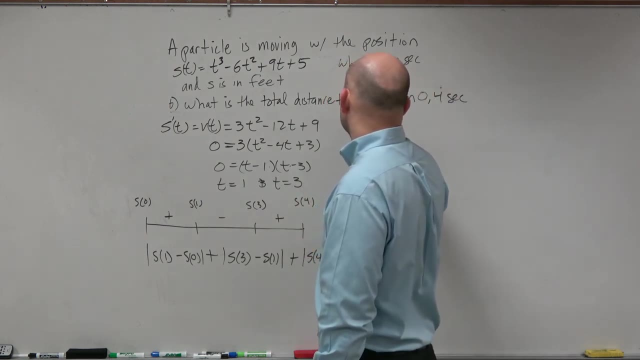 eight miles. So that's what the absolute value helps us To be able to calculate with that. But is everybody OK with this? So now, basically, what we need to do is figure out what all these values are. So s of 0, just plug x of 0 in. 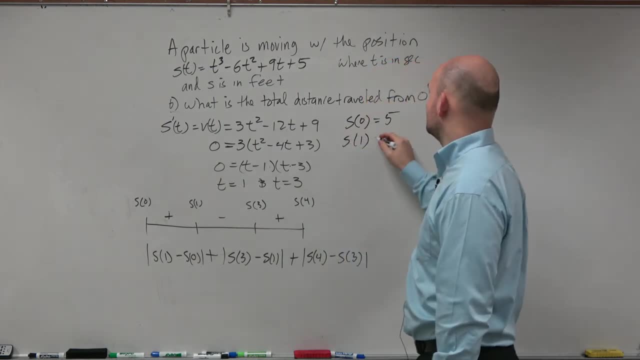 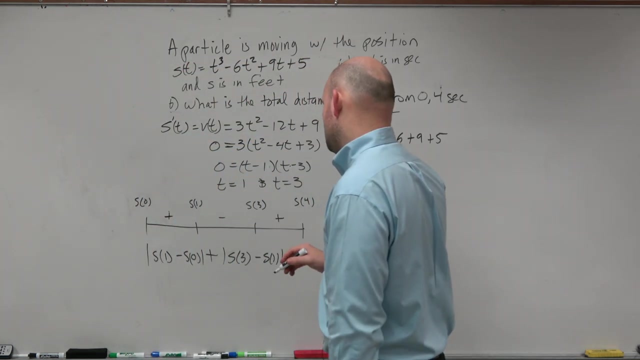 That's going to be 5.. s of 1, that's going to equal- I'm going to do a little bit of math, a little bit more in my head- So 1 minus 6 plus 9 plus 5,, which equals 9. s of 3 plus. 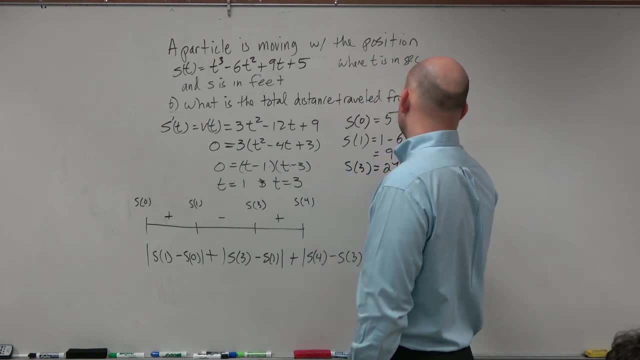 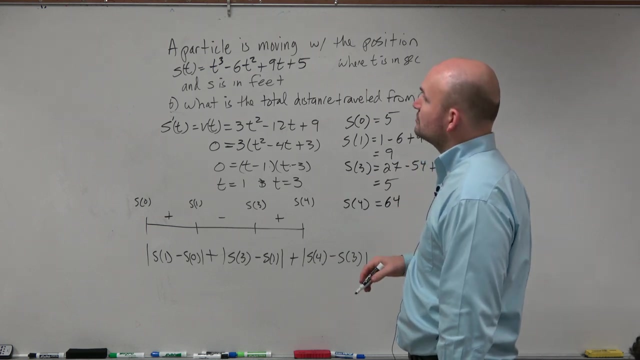 3 equals 27 minus 54, plus 27 plus 5, which equals 5.. And then we've got to do s of 4.. So 4 cubed is going to be 64.. 4 squared is 16.. 4 squared is 16.. 16 times 64.. So that's. 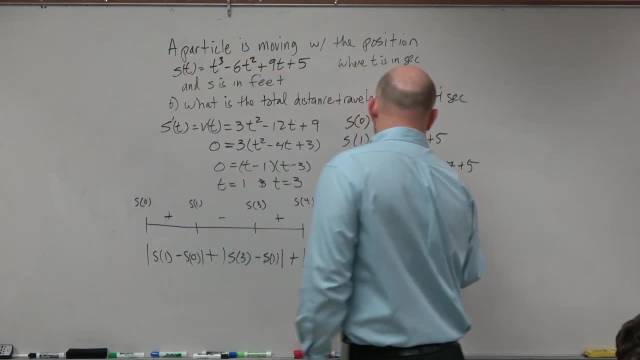 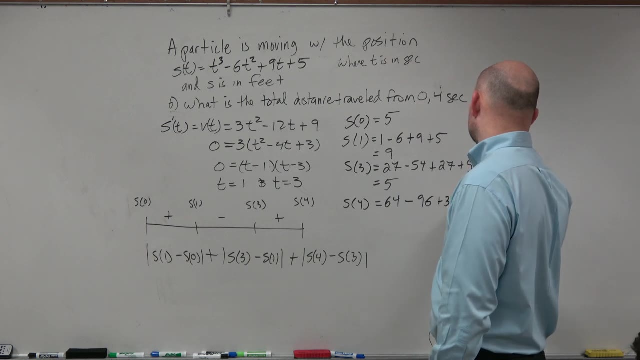 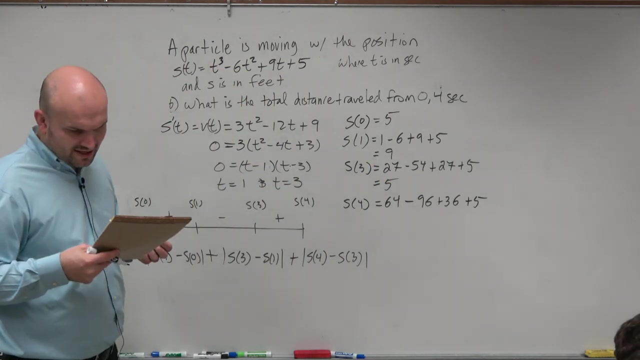 going to be 96 minus 96.. 4 times 3 is positive 36.. And then plus 5.. Check my math in my head to make sure I'm doing this correctly, Because if I got s of 4, it should equal 9.. 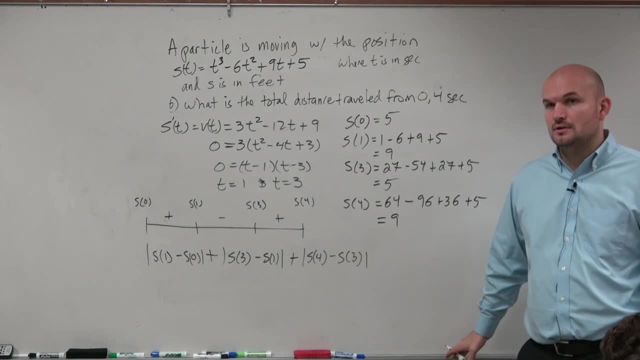 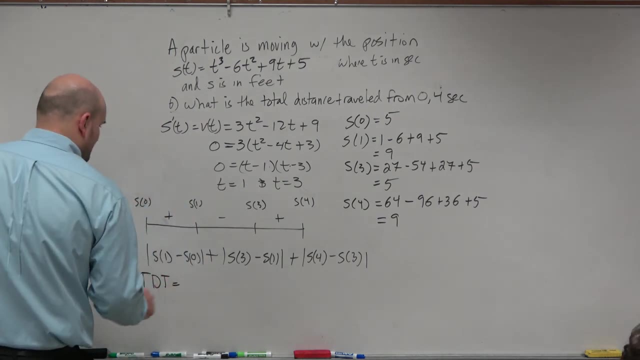 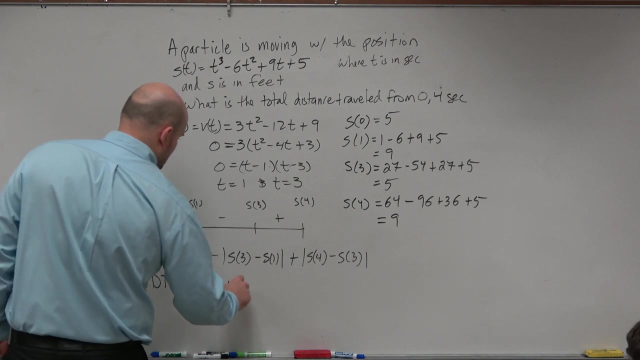 OK, Now to find the total distance traveled is basically just going to be the absolute value of s of 1,, which is 9, minus 5, plus absolute value of s of 3,, which is 5, minus s of 1,. 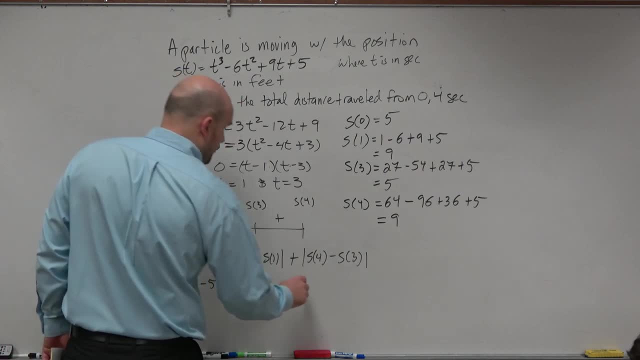 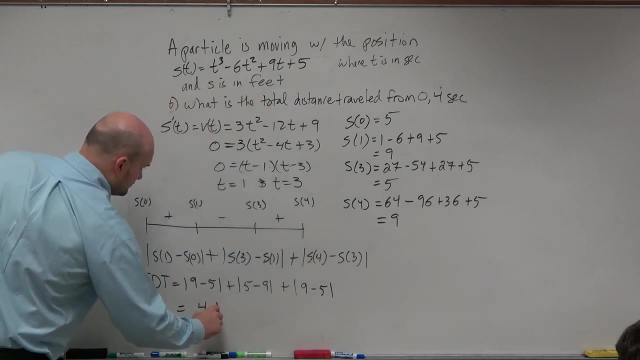 which is 9,, plus absolute value of s of 4,, which is 9,, minus s of 3,, which is 5.. And that is 12 feet. Yes, no, maybe so.